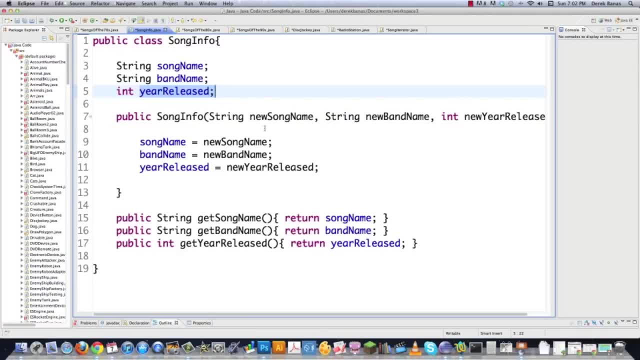 and the release, And on top of that they have to use a function called get best songs that will return the collection of songs. The one thing you forgot to tell them is to use the same collection. So in this situation, the DJ from the 70s is going to send you an array list from the 80s is going 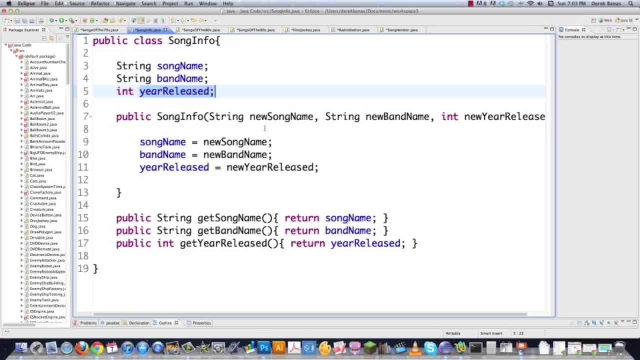 to send you an array of these objects. and then the guy from the 90s is going to send you a hash table. The guy from the 90s is going to send you an array of these objects versus say no, wait a minute. I forgot to tell you I want all of these to be of the same type. 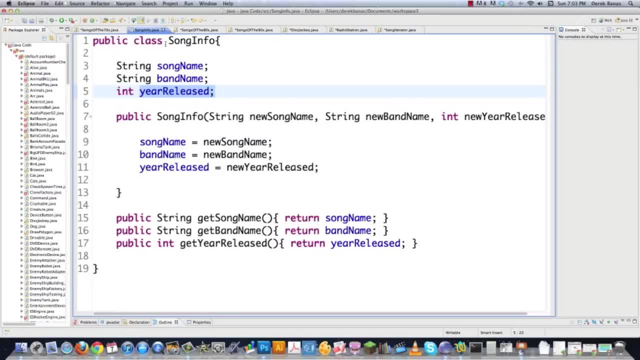 But, being a programmer, you're just going to make things work. So here we go. here is the song, info class, And all the code is available underneath the video, and if you want to 100% understand this stuff, you should go get it. 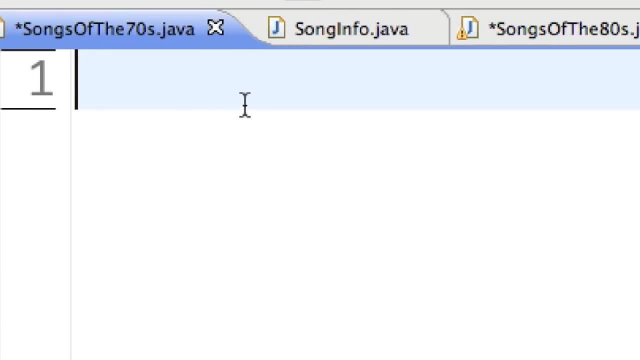 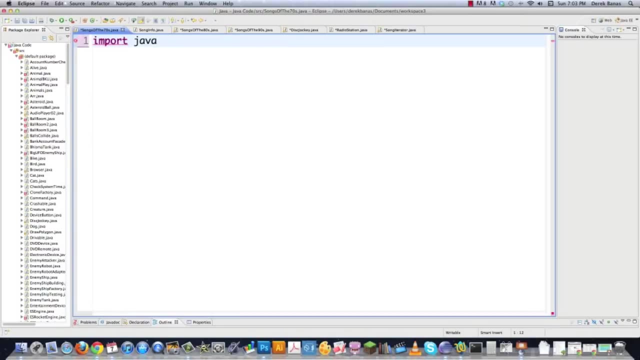 So let's just jump right into it. First thing we're going to do here is go to songs of the 70s And we're going to look at the type of information that we could be expecting from somebody like this. Alright, so they're gonna send us Java util and this guy's going to send us a sp répond. 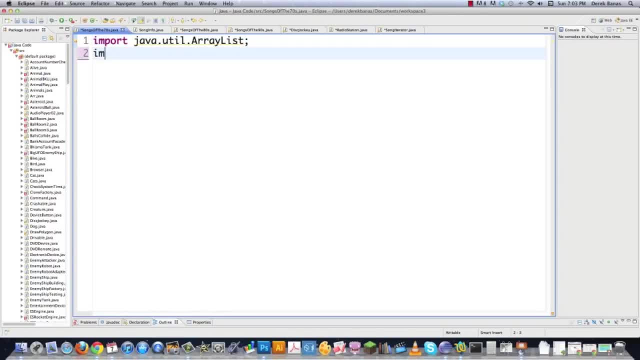 send us an array list. so we're going to need that, and a little bit later on we're going to need the iterator library, so we might as well just put it in here right now. so there we are, okay, and then we're going to create our class. so this is going to be public class songs of the 70s. then we're 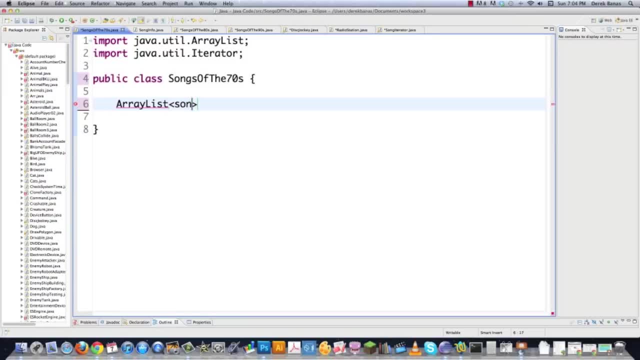 just going to come in here and create an array list and it's going to contain song info, objects, just like we told them, and it's going to be called best songs. of course, make that capital. all right, now that we have that, we're going to create a constructor for this guy. songs of the 70s: this. 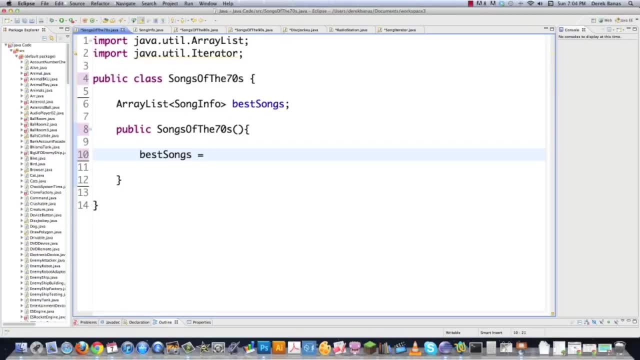 and we're going to go best songs, and what i'm going to do the first time is show you the problem and show you how to force it to work in the wrong way or in a bad way, actually in a very obvious way- and then i'm going to show you how to use the iterator design pattern to do it in a much neater. 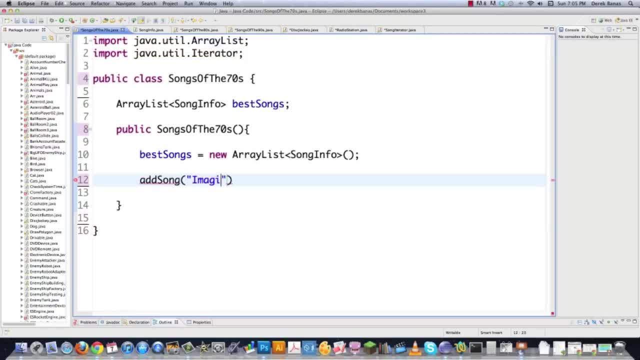 way. so we told them add song needed to be used and these songs are just purely copied, so doesn't have any problem with that. so we're going to create a constructor for this guy. songs of the 70s. this is not anything to do with my musical taste. it's just what popped up on a website, so don't attack. 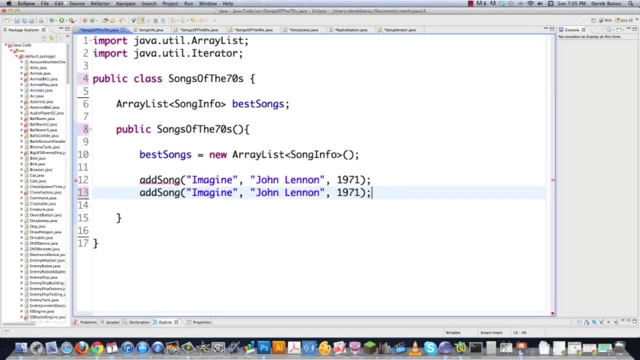 me if you don't like these songs, i'm going to have the add song method, which i'm going to create here in a second, and then we're going to add another song and a final song. so there you go. we're creating the array list and we're adding the song information to this guy inside of the constructor. 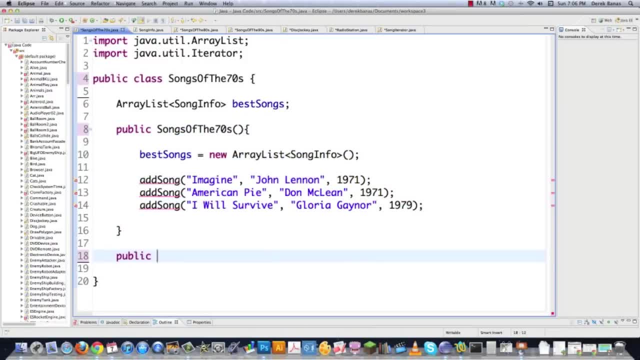 so what do we have to do now? and this is what you're going to be receiving, so we'll go public and you're going to be forced to work with it in a good way. so we need to actually come in here and allow them to call the add song method. song name, string band name, int year release. 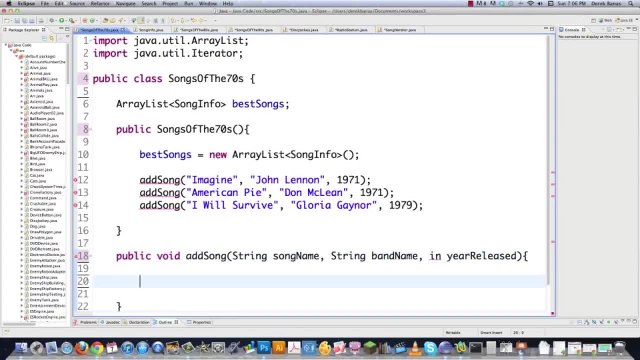 so there's all that information that's going to be sent to this guy and then we're going to have to come in here and go. song info is going to be equal to new song info. song name is going to be passed, band name and year released. so that's. 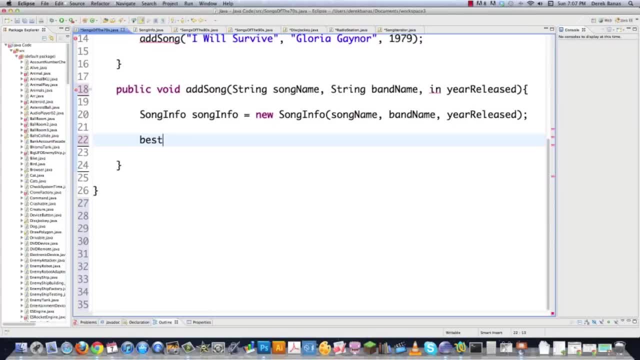 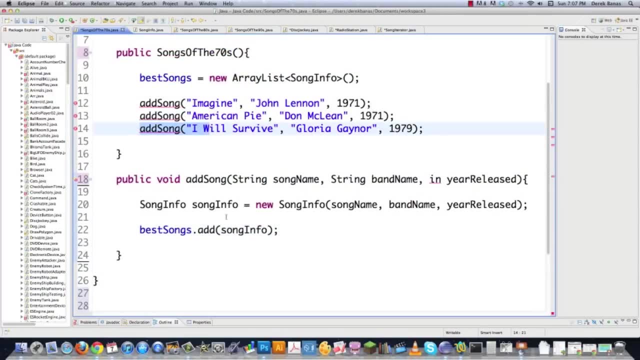 going to create our song info object and then to the array list we're going to add song info. So each time this is called up here, add song- then this is gonna be called down here and then put int there. Then we're gonna do this in. 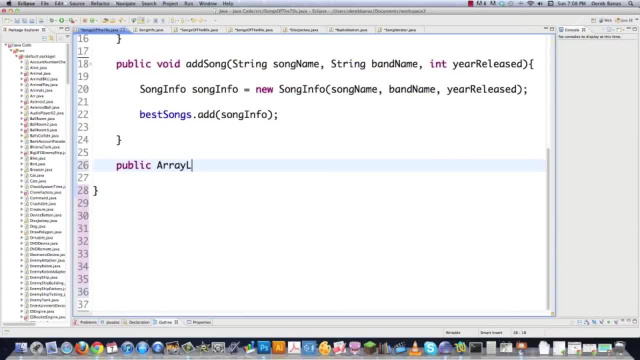 kind of the wrong way. Like I said, I'm gonna show you how to do it in the obvious way and then I'll show you how to do it in a less obvious but a much nicer way. So this is gonna return an array list of type song info and best. 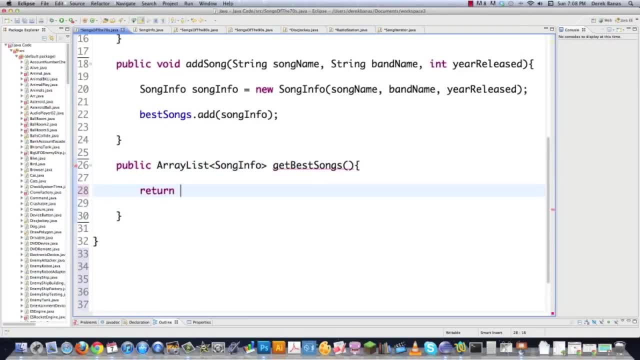 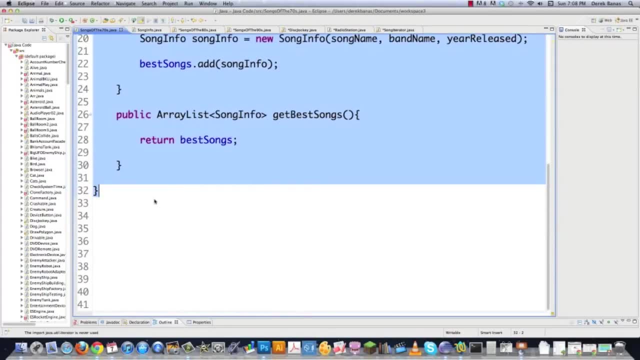 songs is going to return the array list, So just return best songs and that's all we need to do. So it's not messy by any means. It's actually good code, but we have to figure out how to use it for our own situation. So I'm just gonna copy. 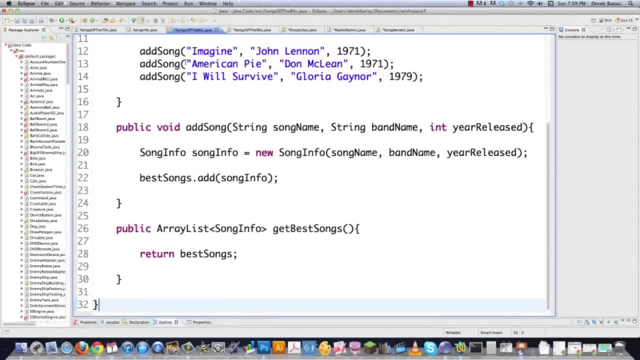 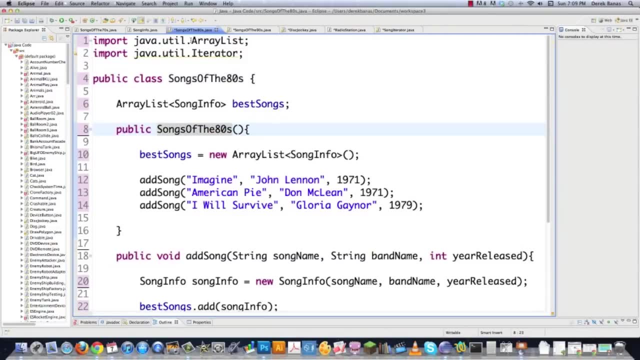 that, and then I'm gonna go into songs of the 80s, bounce in here, paste that in there, and then we're just gonna need to change this to the 80s and this to the 80s, and then this guy's gonna send us an array list or an array that's gonna 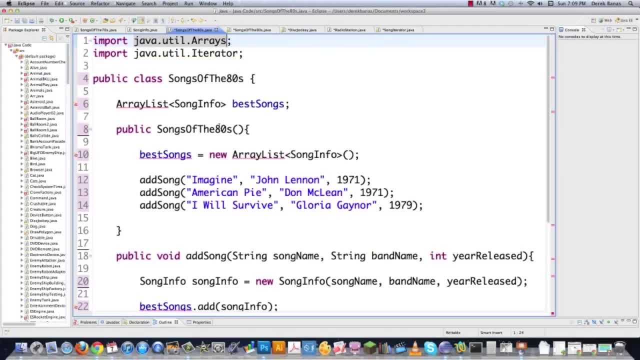 have song info items inside of it. I'm gonna leave all the rest of that the same, and then this guy right here is gonna need to be changed into a song info array, and I'm gonna call it best songs as well, and then I'm going to put an. 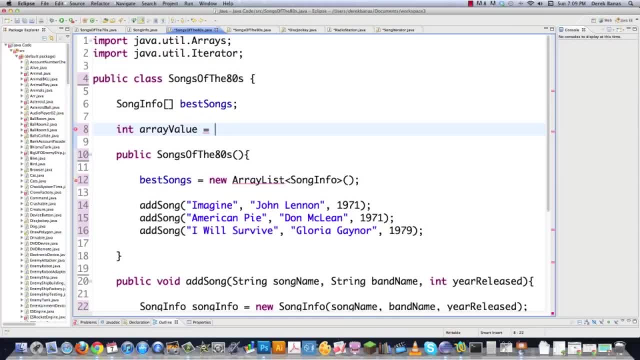 integer inside of here. that's gonna allow us to increment to the next position in our array. So I'm just gonna give that a value of zero in the beginning. Best songs right here. I'm just gonna get rid of this part and go song. 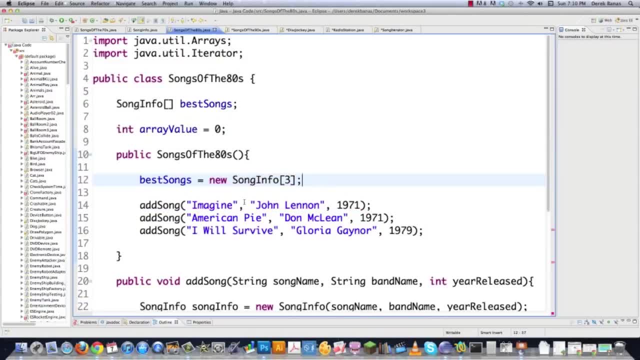 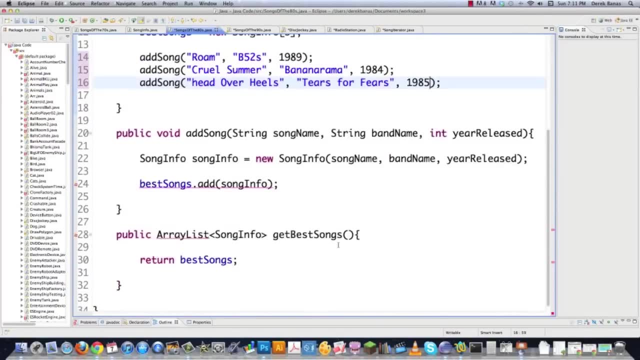 info and say this needs to be three in length, and then all of this is gonna remain pretty much the same. I'm just gonna change the band names here real quick, and there we go. Now we got some new band names inside of there, and then 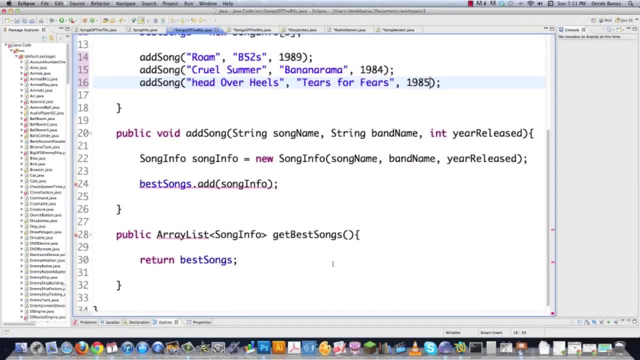 we're gonna have this guy here that's gonna return it to there we go. I put a value named best songs, so that's good. I'm gonna do the same thing, I'm gonna increment that and then we're gonna add a new song. I'm gonna say, in this case, 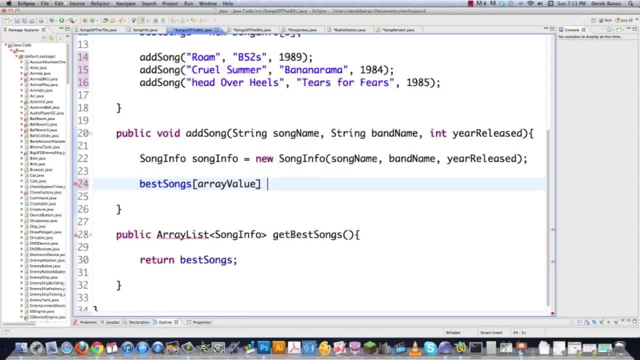 we're gonna add a song info. so now we're gonna go best songs and then go array value same- That's what we're doing there in regards to incrementing that- And then we're gonna add a song object to that? and then go array out value, write that. 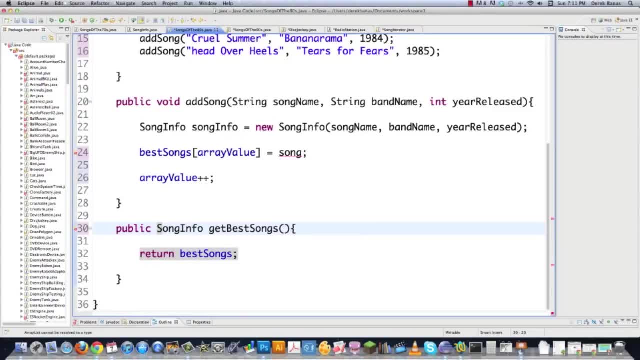 and increment it. So that's pretty cool. And then down here, of course, now we're going to be objects, so we just need to change that and everything else is fine. so we don't need to change anything else and we can just come in here and copy that. and now we're going to go into songs. 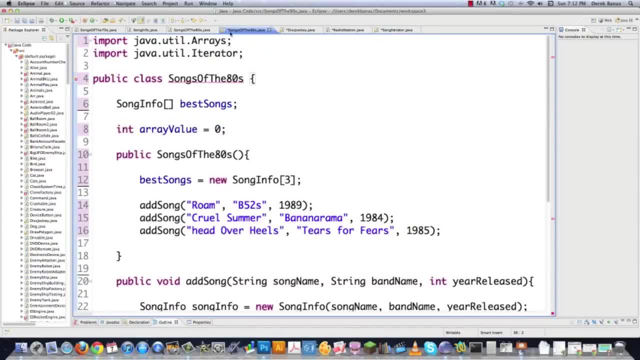 of the 90s. paste that inside of there and that's for songs of the 90s. this guy's going to be sending me a hash table, so we need to get the hash table library there. i'll leave everything else the same. come in here. these guys are going to change because we're going to be holding a hash table. 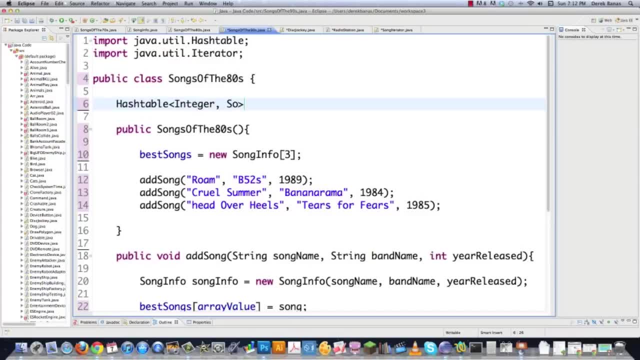 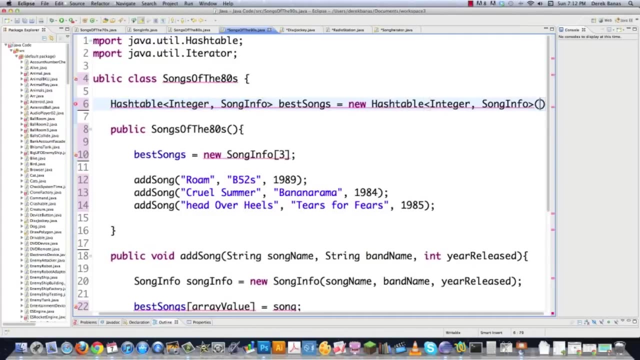 that's going to have an integer object inside of there as the key, and then song info as the actual value- and i'm going to call it best songs, just like before is equal to new. and then it's going to be hash table- exactly the same here as we have on the left side, except we're going to go like this: 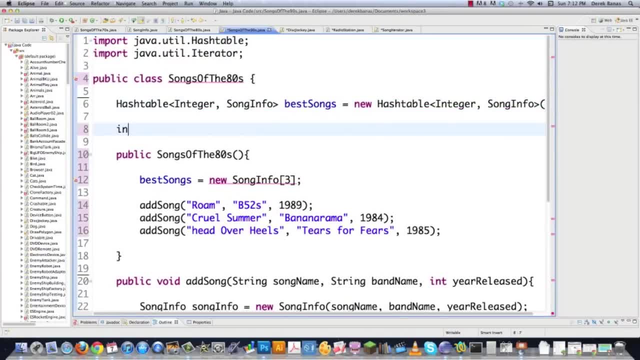 and like that. so that's going to create our hash table for us, and then we're also going to increment the hash key here and i'm going to give it an initial value of zero. so we're going to increment it in much the same way that we 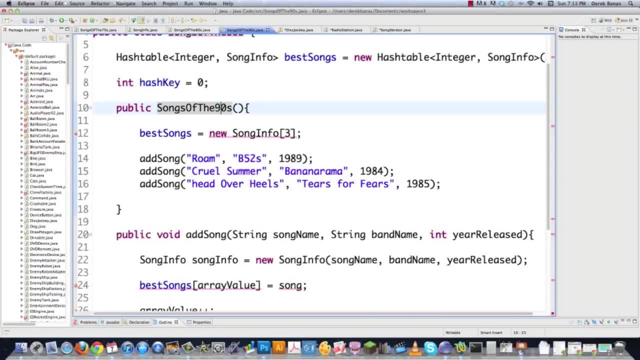 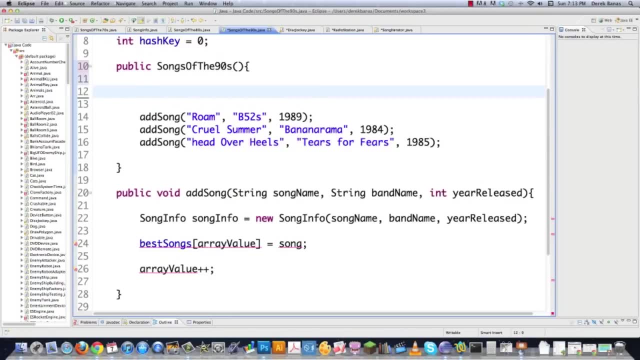 would if we had a hash table. we're incrementing the array and then, of course, we need to change this to songs of the 90s and song of the 90s, just like that. we're not going to need to initialize anything because we already. 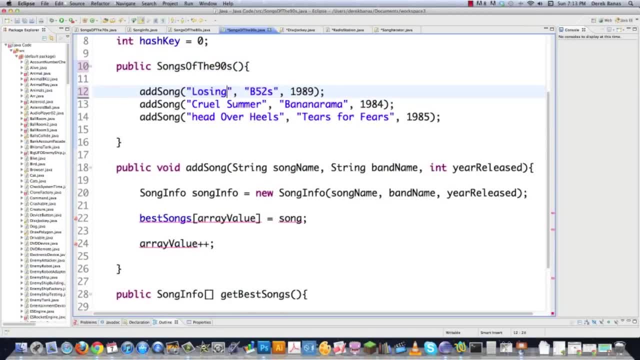 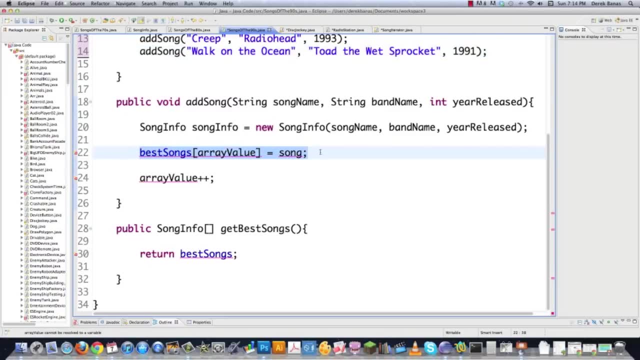 did that, so that's good, and then i'm just going to throw in some more songs and there we are: there's three additional songs, and then down inside of here, we're going to get rid of this guy right here and we're going to type in. actually, i just need to knock off the end. 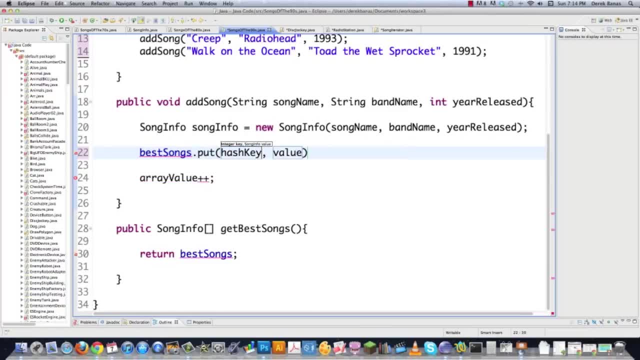 i'm going to call put, which is going to ask for a hash key, and then it's going to ask for the object that's going to go inside of there- get rid of that- and then i just need to increment my hash key and then, of course, down here we're going to be returning this hash key right here. 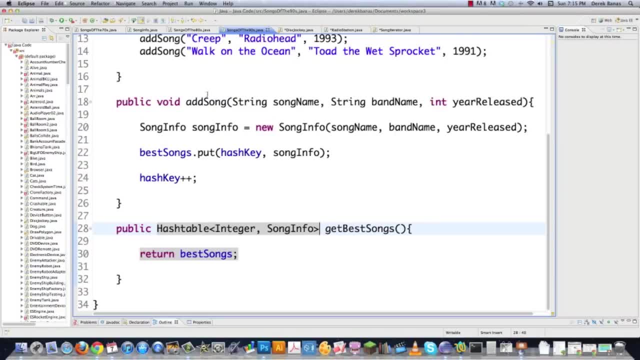 so i'm just going to copy it and there you are, and then we're going to save it. so now we got songs of the 70s, 80s and 90s. so let's go and let's actually take a look at exactly how these are going to work. 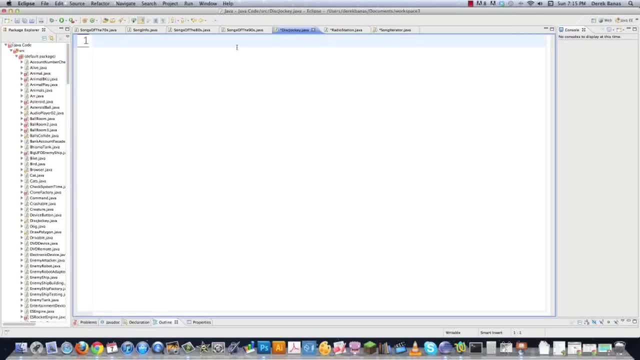 and i'm going to do that in a class called disc jockeyjava. it's going to handle putting all this stuff together, so i'm going to need to get a whole bunch of different libraries in here, till array, list and enumeration and hash table. of course, the code i'm going to show you here in a second it. 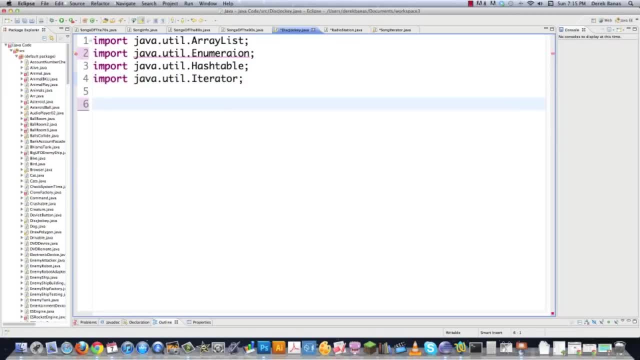 definitely works. it's just not neat and it's obviously not using the iterator design pattern. and then public class disc jockey, and then it's going to go songs of the 70s, and i'm just going to call this songs 70s. and then i have to do exactly the same thing for our other two classes. 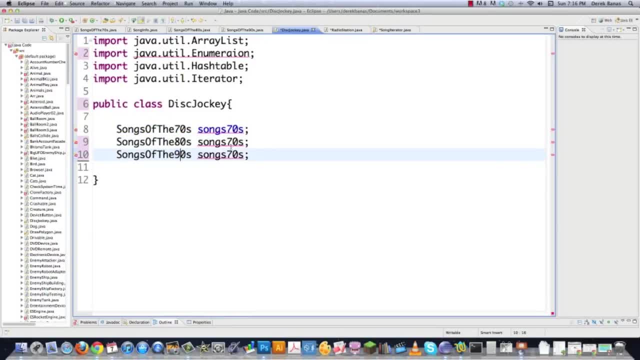 which is the only thing that's different here is the 80s and 90s, and then i'm going to go public disc jockey, create this constructor here, and then it's going to get past all of these values. so let's bounce in there, paste that in there, change that to that, change that to that. 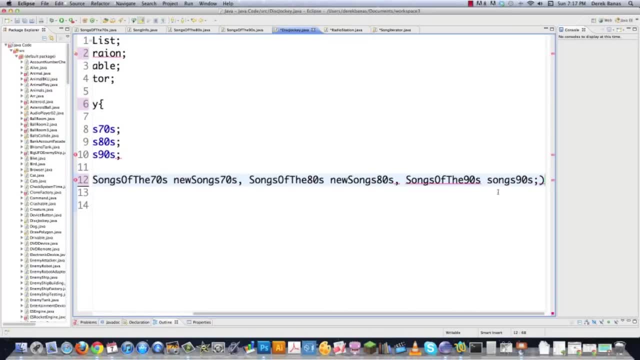 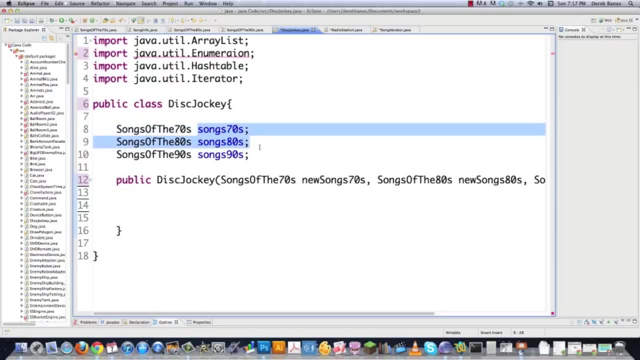 and then i'm just going to call this new, which doesn't matter, i just like to do it that way. there we are, and then, of course, take that there, and then this is going to be really simple. we're just going to go: songs of the 70s, 80s and 90s, paste that in there, and then we're just going. 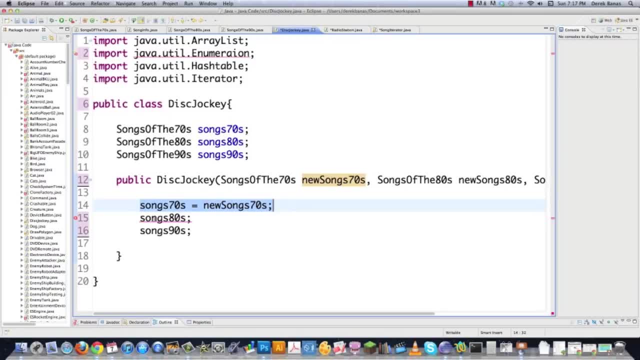 to go equals like that actually makes it a lot simpler just to copy that, paste that three times and then change this to 80s and 90s. so we're just assigning those objects that are being passed over into our own special place inside of our class. so i guess to a certain extent this is kind of a 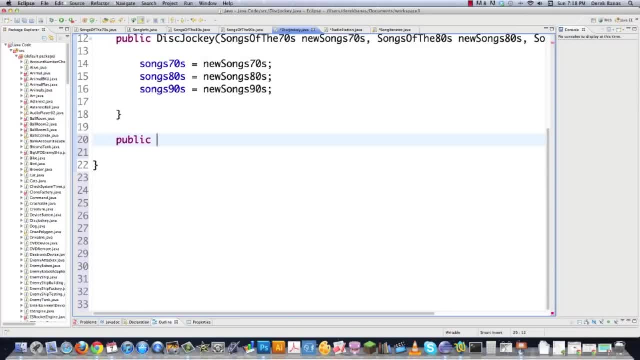 review of using collections. so now we need to implement a method: public void. show the songs and i'm going to show you how you would iterate through all these different types of classes if you didn't know about the iterator design pattern, because all of the song info objects. 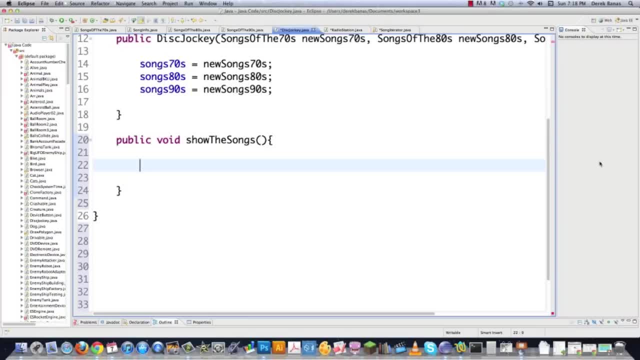 are going to be stored in different collections. everything, of course, needs to be handled on an individual basis, which is terrible, but that's what's going to happen. so i'm just going to call this al 70s songs, that's an array list songs, 70s, dot and then 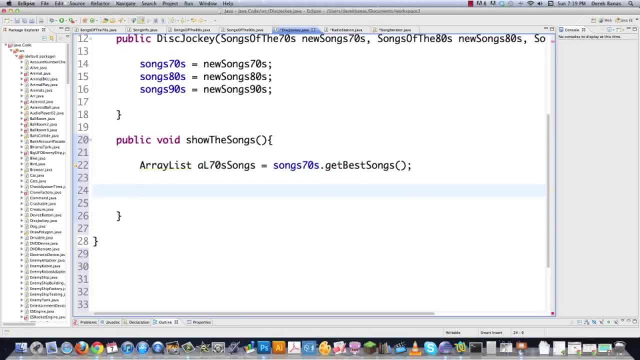 i'm just going to call: get best songs. okay, so we got our array list with all our songs in it. then i'm going to go system out print line and i'm going to say songs of the 70s and then throw a new line in there on top of that, just for the heck of it. and then what do i need to do? well, i'm going 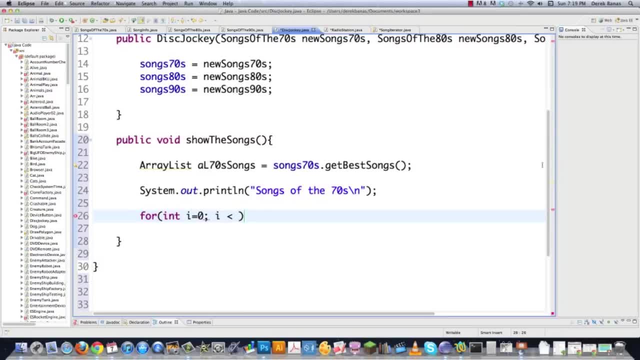 to create a four loopああ here, i is equal to zero, while i is less than gonna get this array list that we just saved everything to and call size on this. since it's an array list, we need to get the length of the total number of objects in the array list like that then. 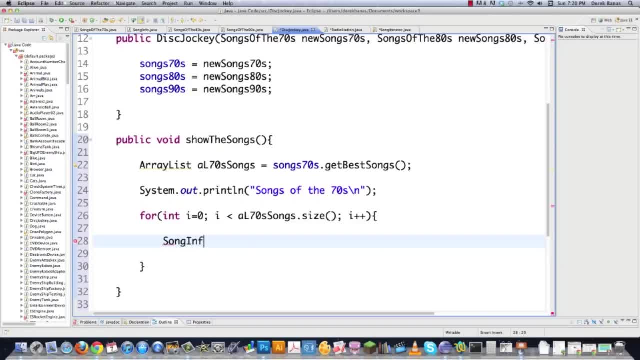 we're gonna cycle through all these and the first thing we're gonna do is go song info- best songs- and then we're going to song list. we need to cast this to a song list. object: array list: 70s songs get and then we have to tell it. 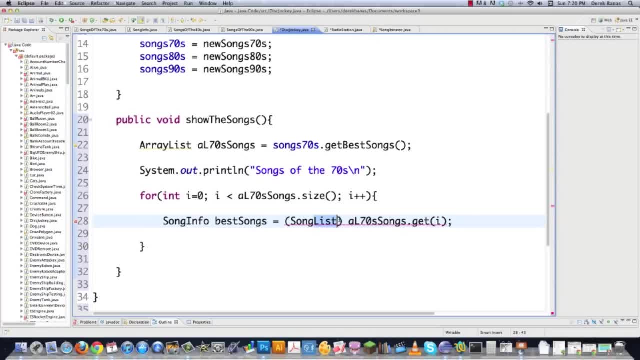 what index to get, which is that's the reason why we have the for loop. oops, this is actually song info, remember, we're using this song info class that we looked at earlier- this guy, all right. so now that we have that, we're just gonna. 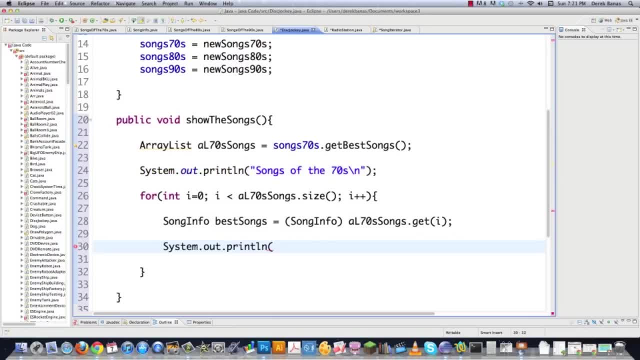 have to print out the name of the song and the name of the band and all this other different stuff. so we just need to go best songs and go get song name which is saved over in that class, and then we're just gonna copy that and then we're. 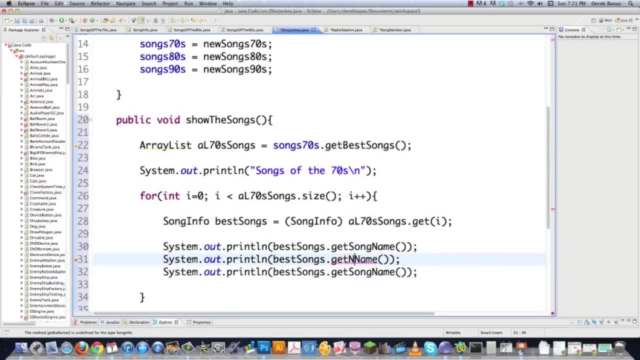 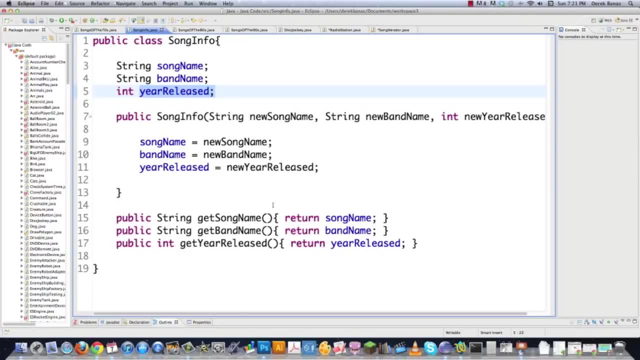 gonna copy this and then, instead of get song name, we're gonna go get band name and then here get release year. so there we go. so pretty easy. giving me a little bit of error, let's see why get year released. okay, so let's just go year. 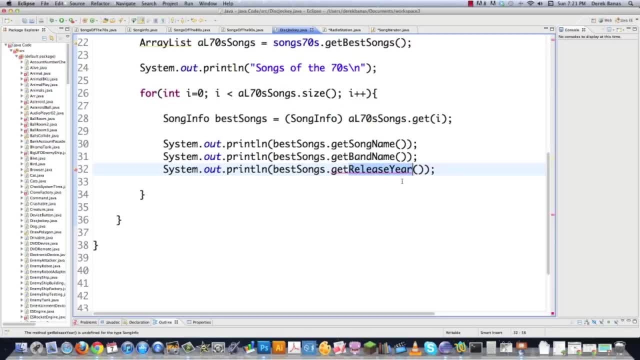 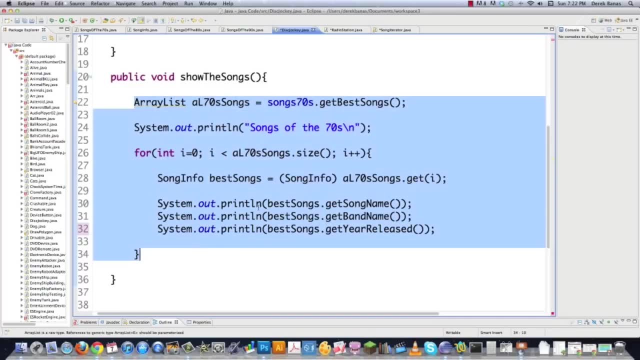 released and jump back over into disc jockey and type in year released and there we are. so there we go. this is gonna work perfectly fine for our array list that is full of song info objects, so now we also. this is the pain in the 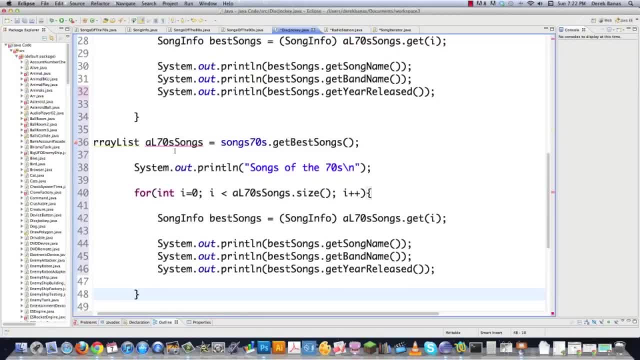 butt part. so you're not never gonna do this after this tutorial. so we're gonna do this after this tutorial. now we need to do a similar thing, except this time we're going to do it with an array. this is no longer an array list, it's going to. 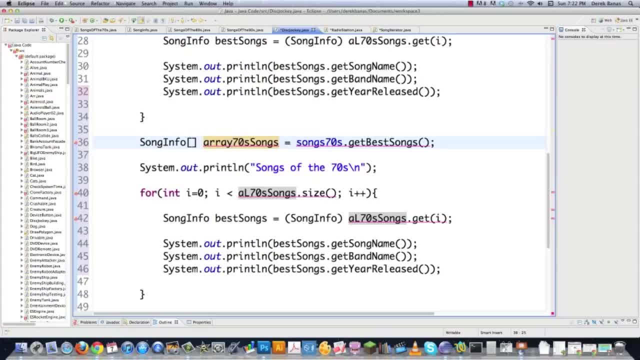 be song info like that, and we're just gonna call this array: 80 songs, change this to 80s, get best songs, all that's gonna work. still. change this to 80s and then this guy. we're gonna be going through an array now, so paste that in. 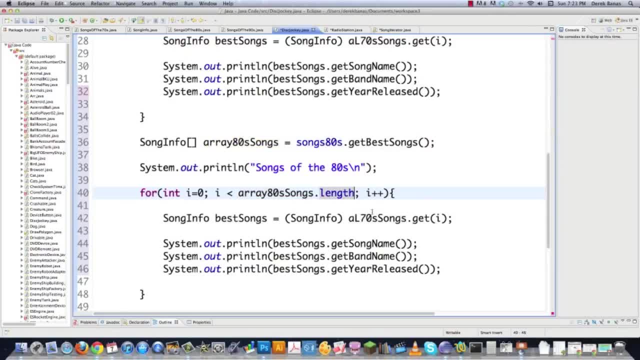 there, and then this time we're gonna call length, because that's what you do with an array, and then down here we're gonna leave this song info, best song songs- except this is going to be this guy right here, so let's just copy that. 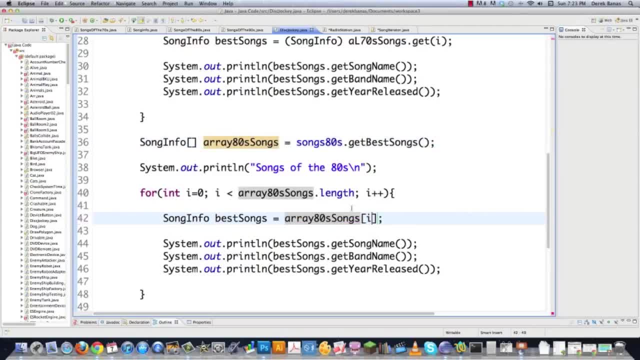 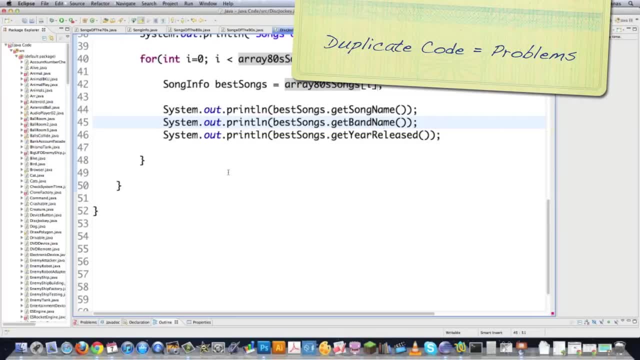 paste that there and then this is going to be I, so get all that, and then everything else needs to say the exactly the same. so in general, it's good code. it's just, you know, this is too much, so then we got to do the same exact thing. 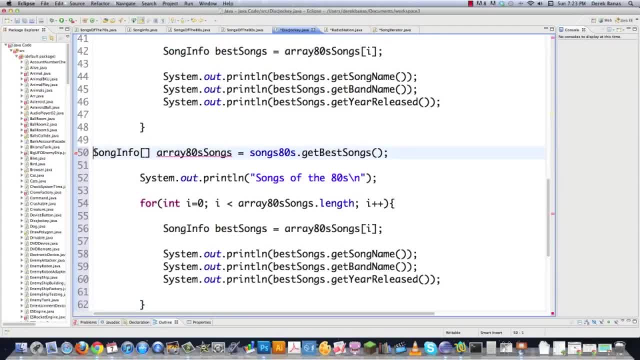 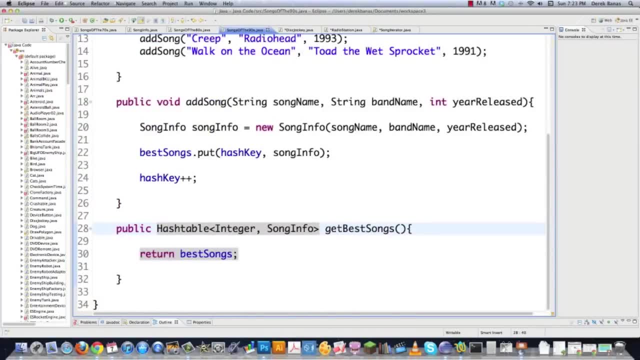 for hash tables, and we shall so paste that in there. now we're gonna see how to cycle through hash tables with objects in them. so what are we gonna do? we're going to first off, we're gonna jump over to songs in the 90s, we're gonna copy. 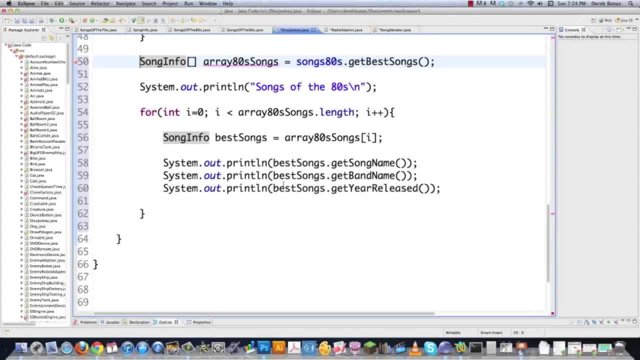 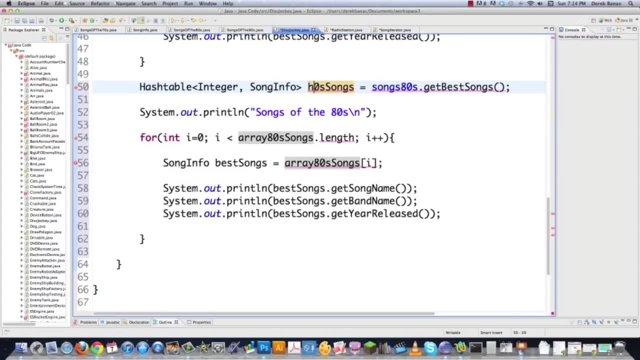 this because I don't feel like typing all that out again and then jump back over into disk jockey and then this is going to be that very specific type of hash table and then here we're going to call this ht 90 songs and everything else is going to be the same on that line, same good code, just. 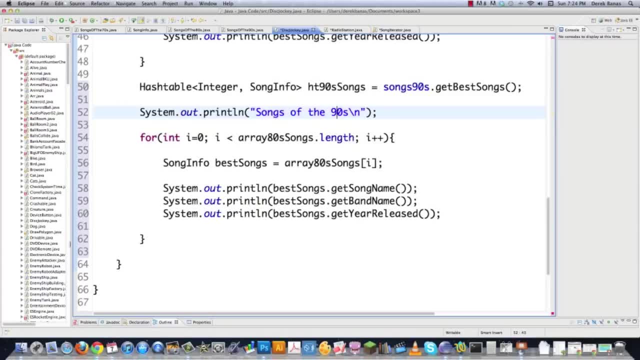 messy. this is going to be changed to songs of the 90s and then the for loop down. here, instead of using this stuff, we're going to use an enumeration that's going to hold our keys for us. so remember we were using integers and I'm just going to call this: e is equal to ht 90s songs, and then we're. 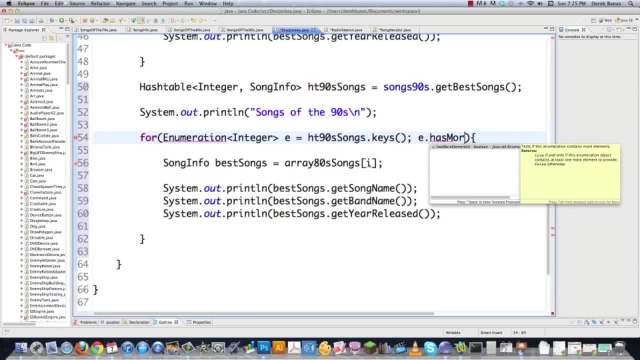 going to go key. now I'm going to go e. so while I have more elements in this hash table, I want to continue this looping. so that's all that's going on there. this is going to stay the same, except- and we're going to go- ht 90 songs. 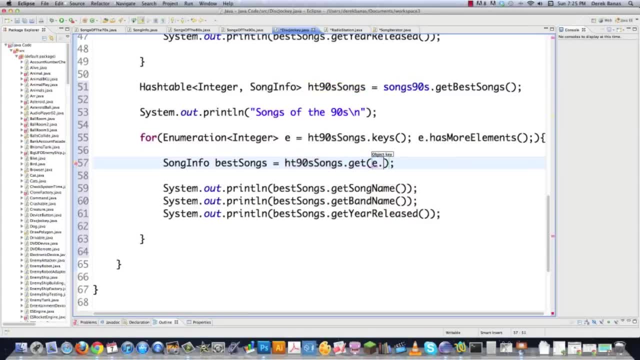 basically in there, and then we're going to go call git and then e. we have to give it our key, which next element is going to have the value for our key, and then everything else can be exactly the same. so there we go. it's kind of long-winded, but it's still good code. so you know, you can't really. 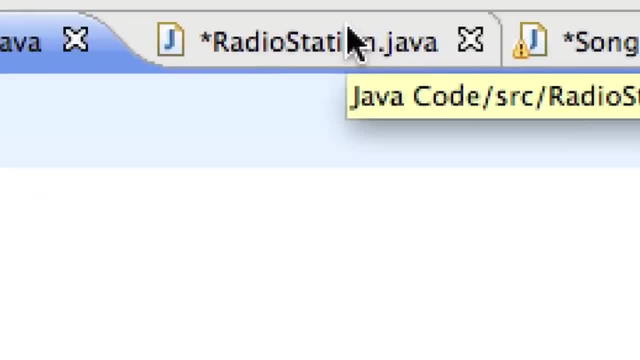 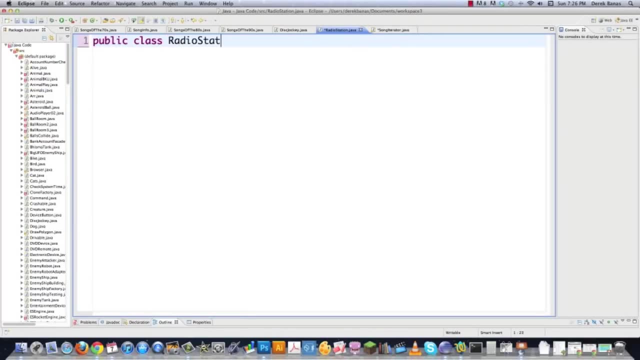 complain. so now let's file, save that and i'll show you how all this is going to work. i'm going to go into radio stationjava and this is going to work very easily. we're going to go public class radio station and then we're going to go public static void main string, there's that args and 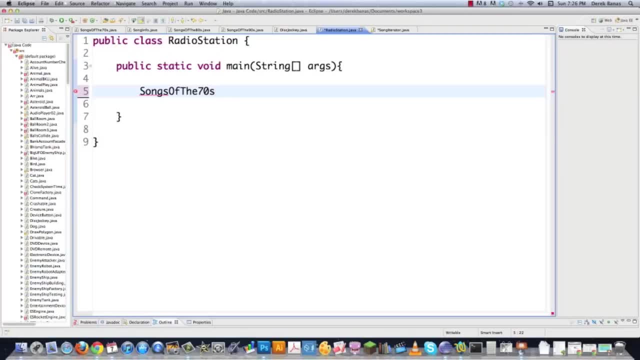 then i'm going to go: songs of the 70s songs- 70s is equal to new songs of the 70s. so we're going to create this object here, right like that. so very simple, still pretty neat. and then we're going to do exactly the same thing for songs of the 80s as well as the 90s, and there and there. there we are. 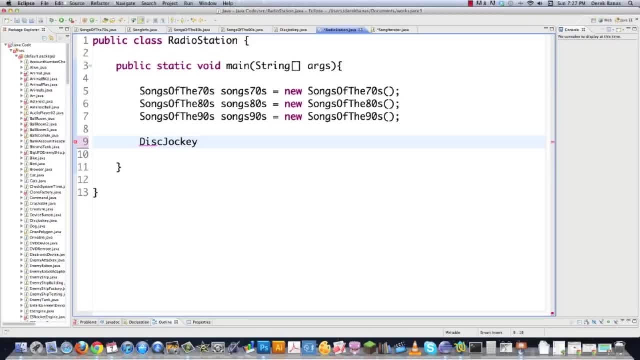 and now, if we want to go to the radio station, we're going to go public static void main string. we're going to go disc jockey and we're going to say our disc jockey has the name mad mike. we've got a new disc jockey and we're going to send him over songs of the 70s for him to play songs. 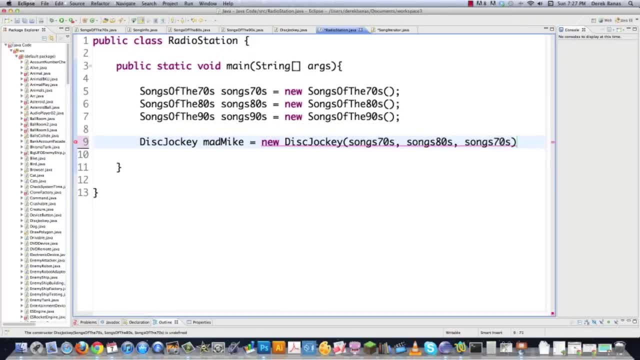 and this is going to be 80s and then this is going to be 90s. so pretty simple. and then to get mad mike to play these guys, we're going to go, mad mike show the songs and if we did everything right and we run this, it shall work. and there you can see it did. okay, see it prints out. so we're going to go. 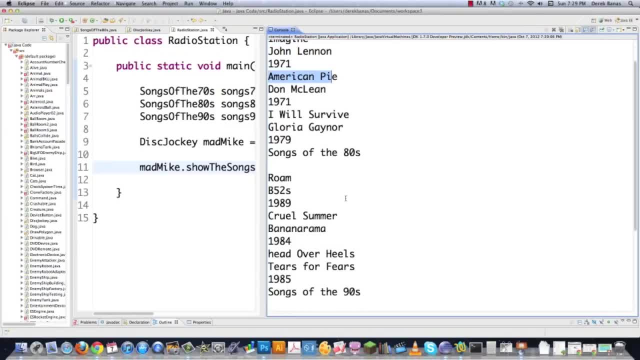 songs of the 70s. and then you get imagine john lennon, american pie, blah, blah, blah, blah, blah, blah, songs of the 80s and room and all these other different things and songs of the 90s. so hey, it works. so why complain about it? well, the reason: why is it's possible to make it work? 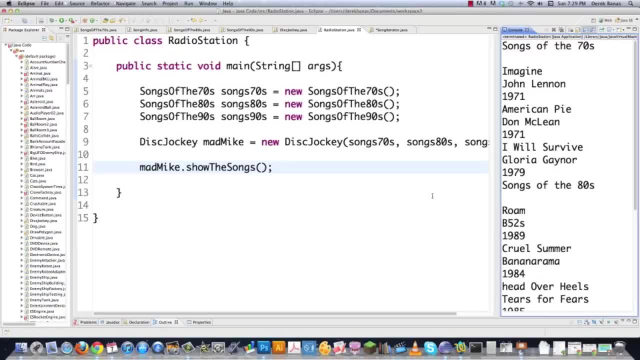 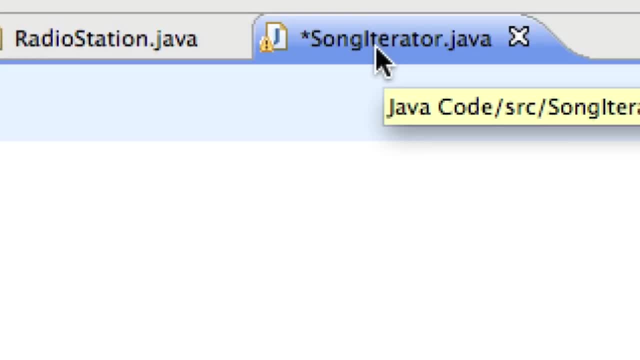 that much better. it's really the difference between being a great programmer and an okay programmer, and how we're going to make this work beautifully is we're going to create ourselves a new interface and it's going to be called song iteratorjava. this is going to allow me to refer. 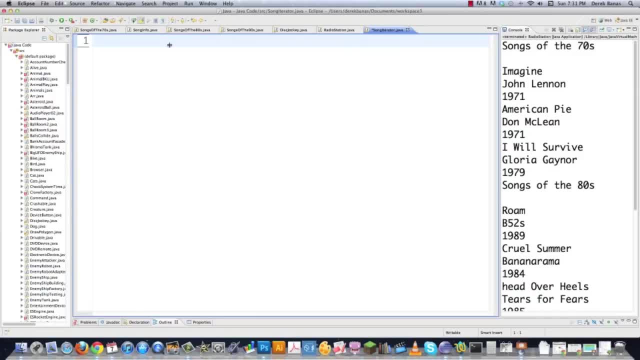 to any of the songs that i've played. so we're going to create a new interface and it's going to everything as a song iterator. every single one of these previous classes that we created will now be referred to as one, so the first thing we need to do, of course, is import our java iterator library. 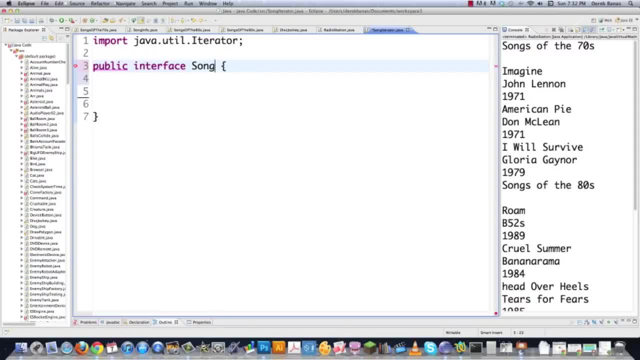 and then we're going to go public interface- song iterator, and then we're going to go public iterator. this is going to be the class that has to be created and it's going to be called create iterator. not much work to put into creating something that's going to make everything really. 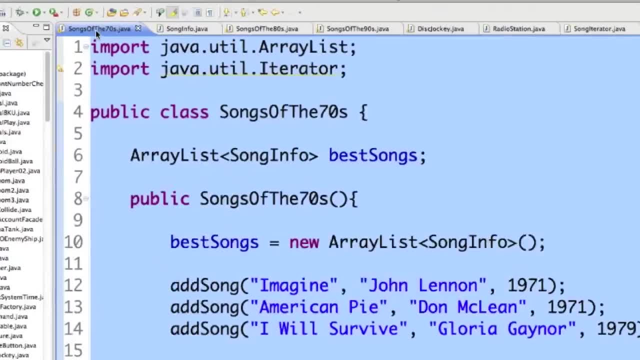 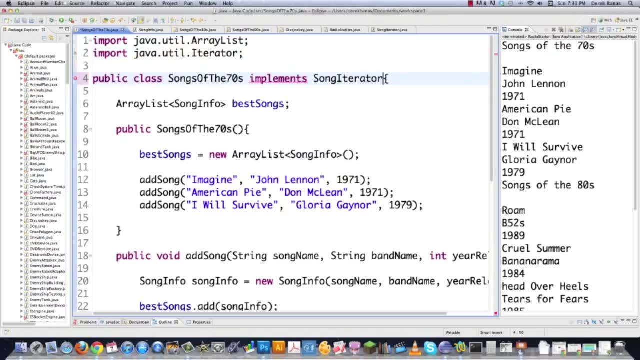 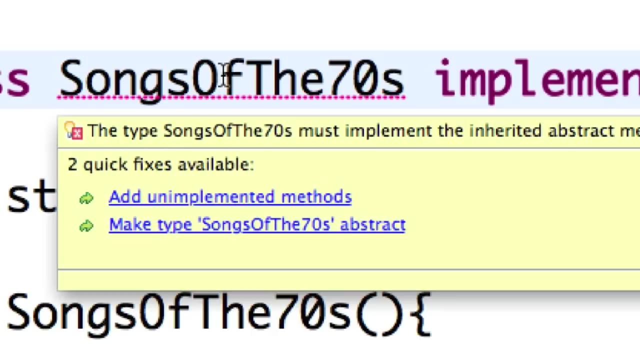 really cool, so let's file, save that and then make all this work. we're going to jump into songs of the 70sjava and we just need to go implements song iterator, right like that, and then it's going to give us an error message. songs of the 70s is going to say, hey, you need to bring in some unimplemented. 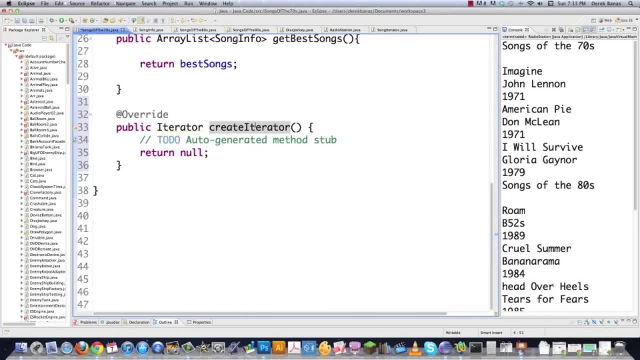 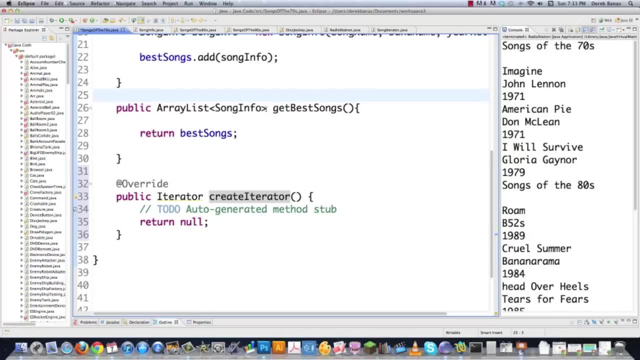 methods and we shall click on that. then we need to scroll down right here and we need to just pop out an iterator that's going to make it easier to use this guy, and before we do that, we can come in here and say, hey, we don't need this. 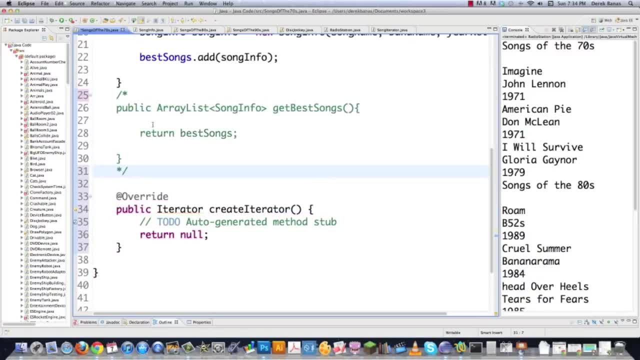 anymore, which is a mess. we don't want them to send back an array list because that's not neat and that's not good coding. so there, that's gone. and then come in here to public iterator, and then what it's going to do is return an iterator here. it's going to allow us to easily bounce through. 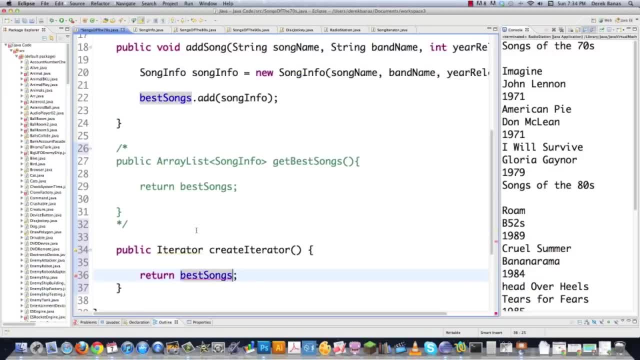 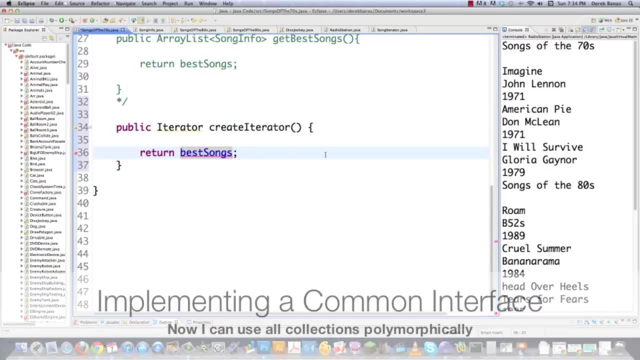 everything we got here and we're going to go return best songs. and what's best songs? best songs? you see it everywhere. this is the array list, see: best songs. this is the array list. and then all we need to do is, instead of bouncing back in array list, we're going to go ahead and 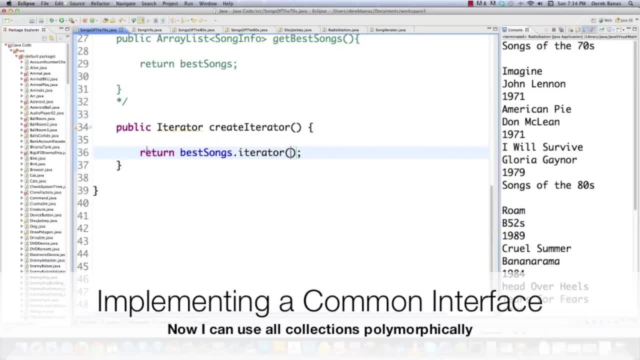 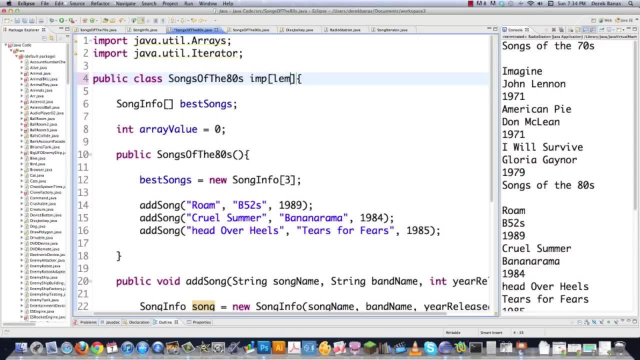 we need to bounce back an iterator and do that just by doing that, and there we are. well, we did a lot. okay, pretty cool. so now we need to do the same thing with songs of the 80sjava. so we're going to come in here and go implements song iterator. see another thing that's great about. 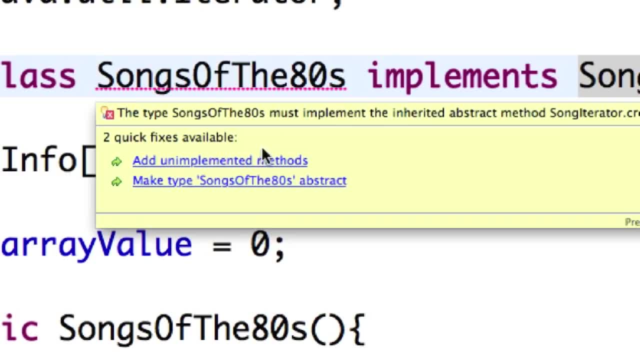 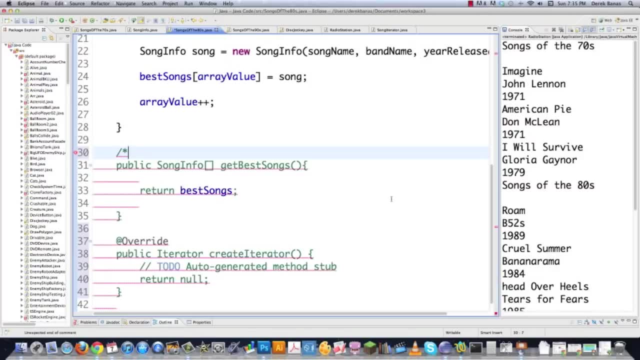 this is- we're not changing that much code- always a good thing. come in here, add unimplemented methods. bounce down to the bottom of the screen. come in here, remember where we're sending back an array. well, we don't want to do that. instead, we want to send an iterator, and there we are, so got rid of. 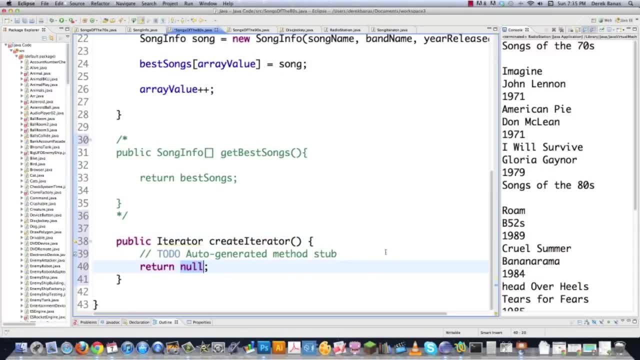 this, if you want, and down here, instead of sending back an array, like we were doing before, we're instead going to send back an iterator, of course, and to do that we go raise as list and then send it best songs, which is the name of our array inside of here, and then call it iterator, like. 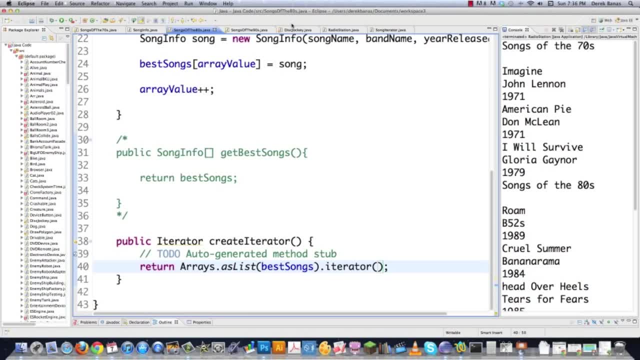 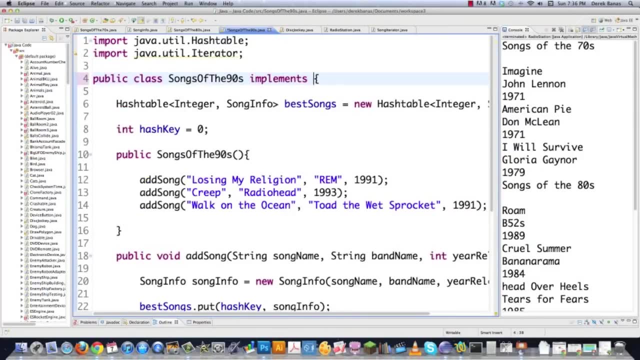 that. and there we are: now it's an iterator, and now at least it's sending back the iterator. so let's save that now. let's go fix songs of the 90s. see how easy this is. and what are we gonna do? we're going to go in here and we're going to type in values like that and then we're going to do is: 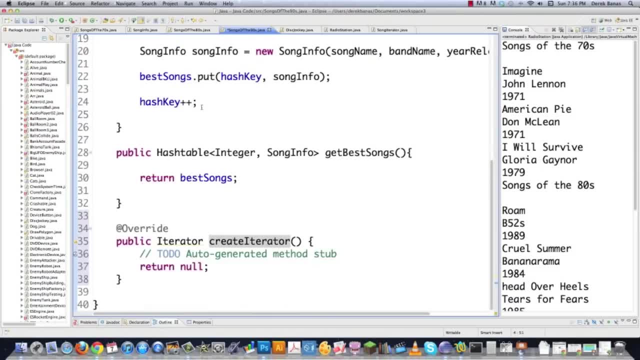 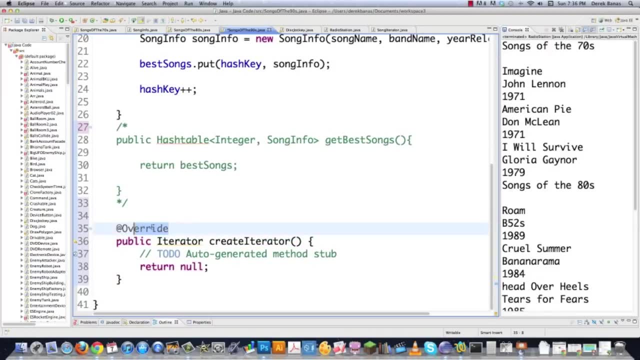 we're going to type in values like this and it's going to say: hey, you need to implement some stuff, no problem, go implement that scroll down. okay, we don't want to return a hash table anymore because that's not good and let's get rid of that. of course, you delete it normally and then down here. 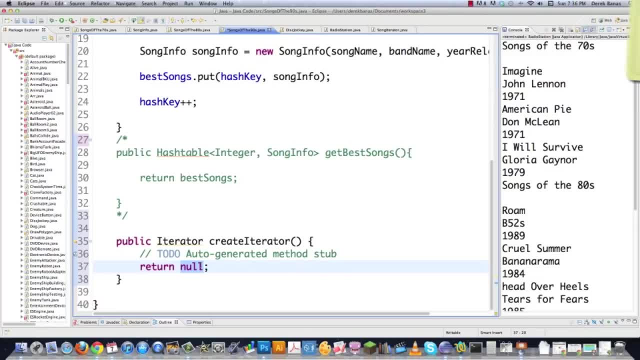 now we need to send back an iterator for the hash table instead of a hash table, and to do that, we're just going to come in here and go best songs, which is the name of my hash table, type in values like dot iterator. i'll save there. you are done so. now what's left to do? since that was so simple, well, 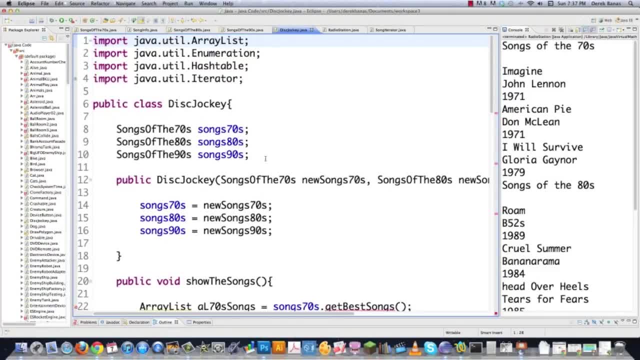 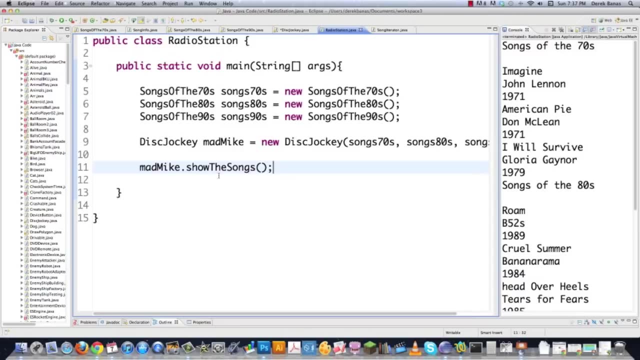 of course, we need to go into disc jockeyjava and save or change everything we got here. so now, instead of passing this stuff here, we're going to create song iterator. see, we're going to refer to everything that implements the song iterator interface as a song interface. see, we're able 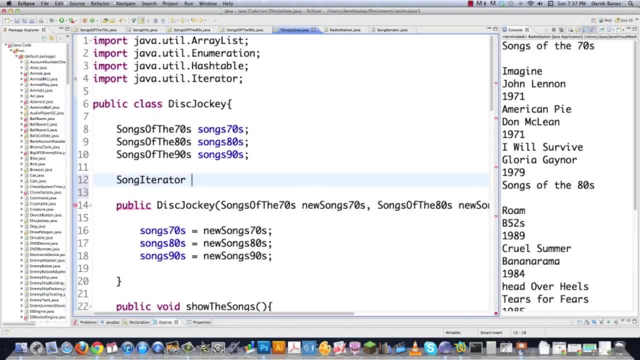 to refer to everything as if it's the same thing- always a good thing. so we're going to refer to it as a song iterator and i'm just going to call this iter 70s songs. okay, got that set up copy and then here we're going to go 80s and we're going to go 90s. see, we're going to refer to. 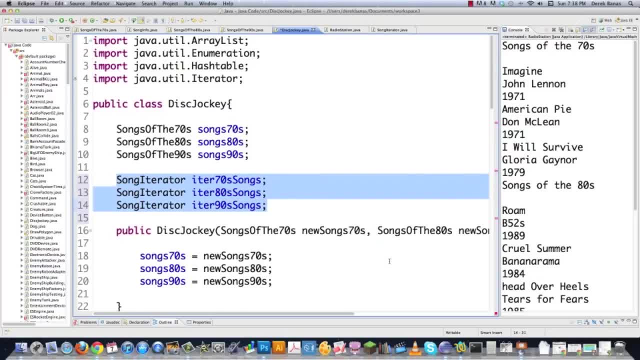 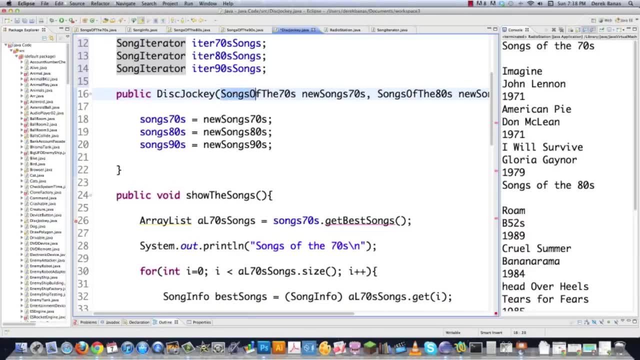 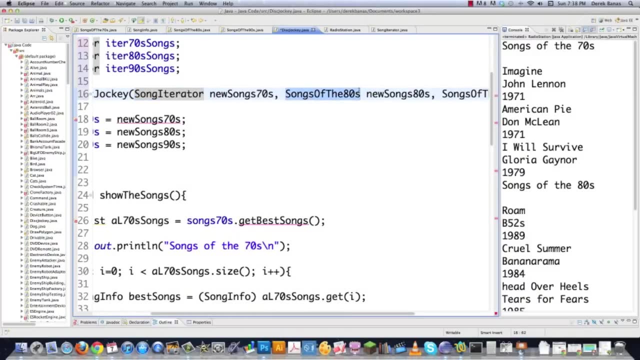 everything now as a iterator, which is always great, and then we need to get rid of this guy altogether. so let's just delete it, the disc jockey. or, better yet, let's just change this from songs of the 70s to song iterator. so copy song iterator, like that. and this is going to be. 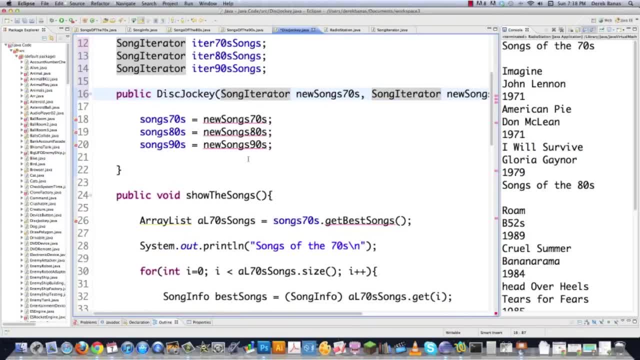 song iterator, iterator, and this is gonna be song iterator. There that goes. I'm gonna leave everything else to have the same name, and then song 70s is going to be new song 70s, and then we're gonna need to change song 70s to iter 70s, right there. 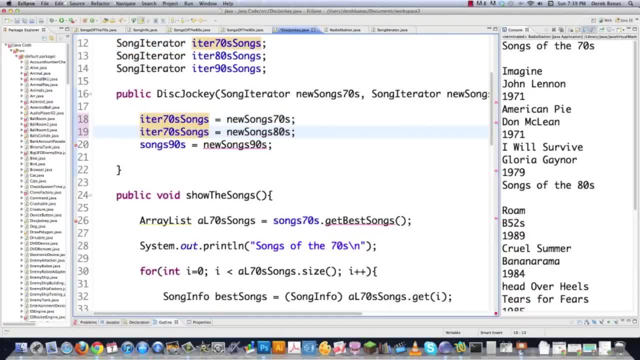 So this is an interface, and then this is going to be the interface that's going to represent the 80s, and this is going to be the interface that represents the 90s. So there we are. Now we got that set, and then I'm just gonna skip this whole. 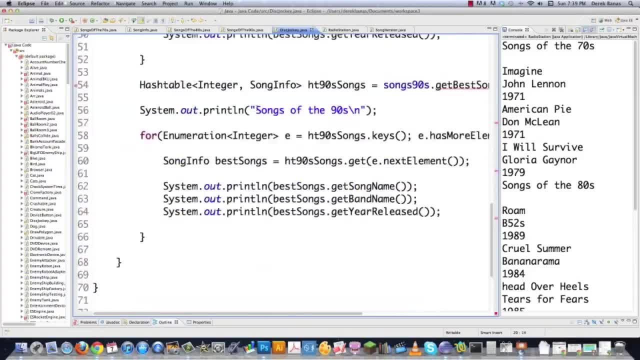 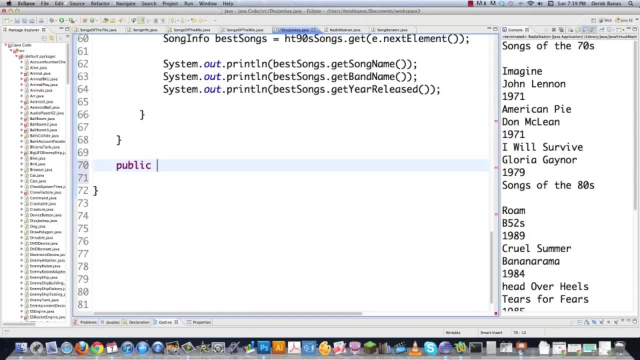 thing, show the songs. So let's just leave that there in the code so that you can look at it later and see the way not to do this. And now what I'm gonna do is treat everything as an iterator. So we're gonna go public void and I'm gonna call. 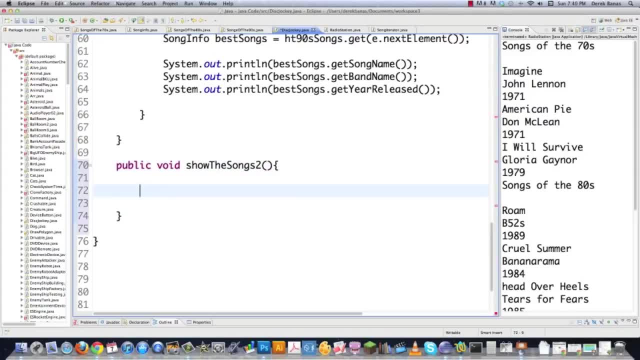 this show the songs to just for brevity. and then I'm gonna go: iterator songs 70s is equal to iterator 70s songs and call: create iterator. like that, Pretty simple Copy that. Now we need to do the same. 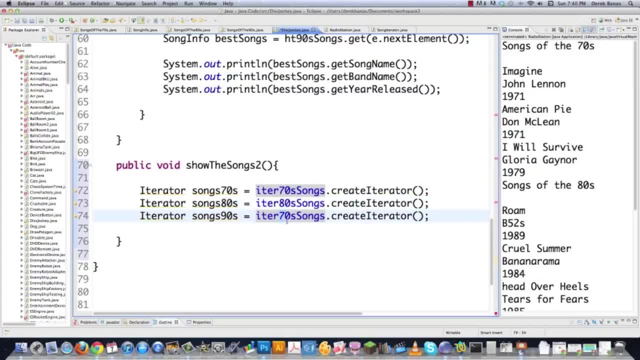 thing for the song iterator. Now we need to do the same thing for the song iterator. Now we need to do the same thing for the song iterator. Now we need to do the same thing for the 80s and the 90s- 80s, 90s. there we are Done, So now we have those all set up. 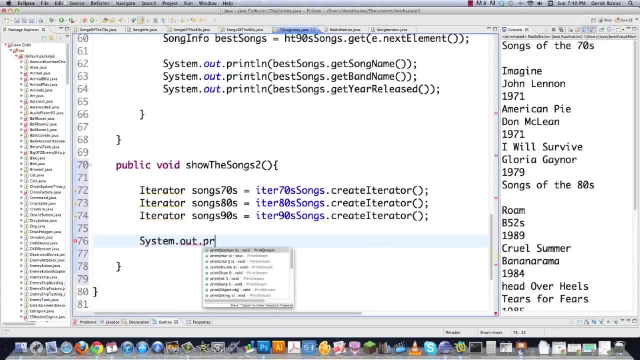 and watch how easy it is to now print everything out properly: Print line. I'm gonna go songs of the 70s, throw in a new line and then to print out. print the songs which I'm gonna create here in a half a second. Songs 70s, right like this. 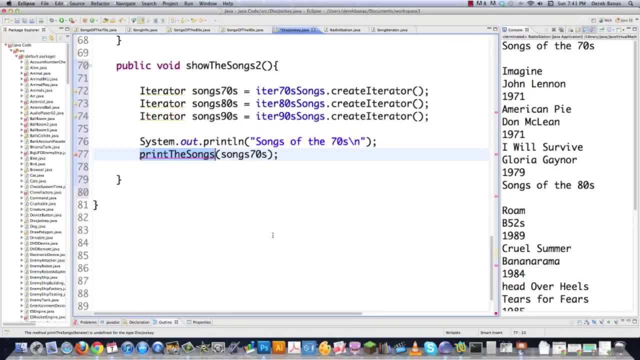 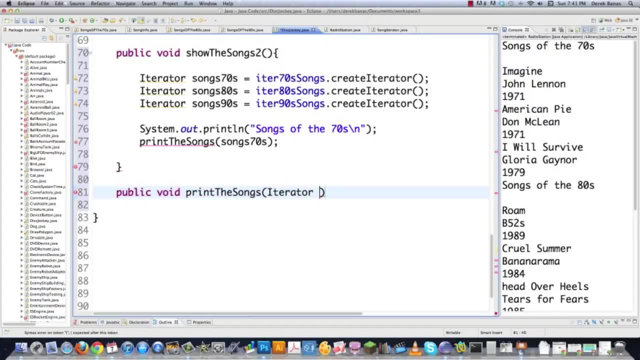 Change that to uppercase, and actually I'm gonna do it right now, just so you can see it here all on one screen. We're gonna go public void, print the songs and it's going to get an iterator sent to it- Iterator like that. 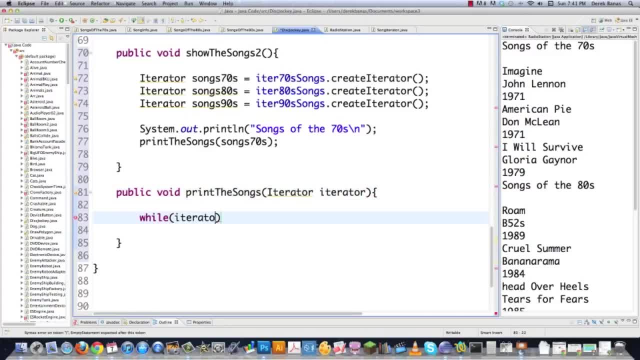 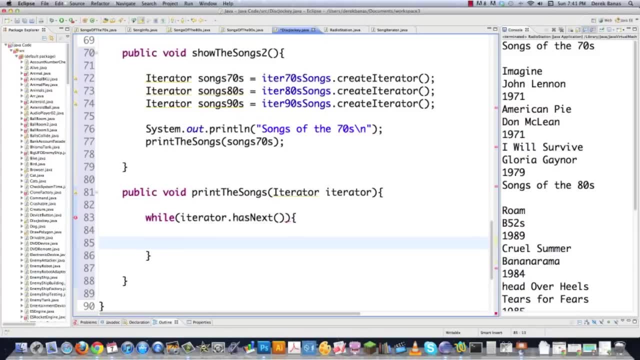 and then we're gonna go while See, we're gonna be able to treat every one of these, even though they're different collection types, as if they're one. So as long as we have more elements in our iterator, we're going to print out. 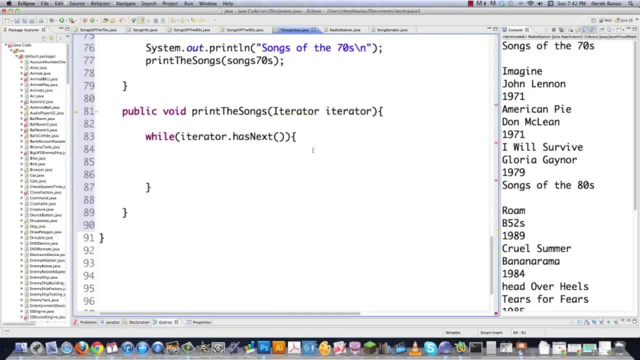 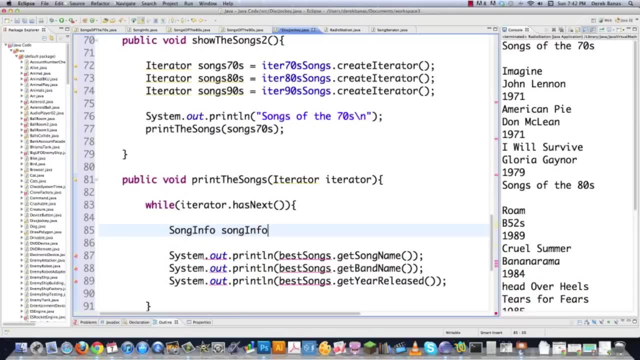